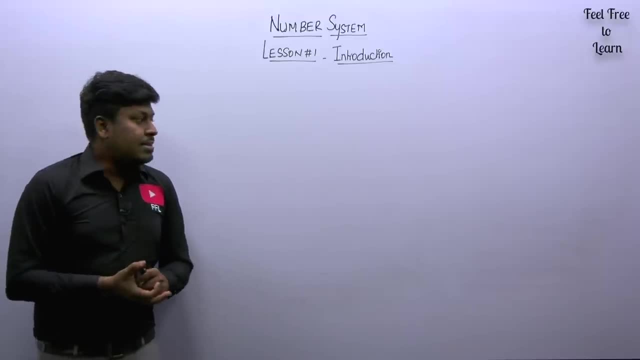 how to solve the question right. So listen here. in this video, I'm just going to teach you the easiest way to learn. I'm just going to draw a chart here so that you can able to learn all the concepts easily by only the chart. So now let me move on to the chart that is based on number. 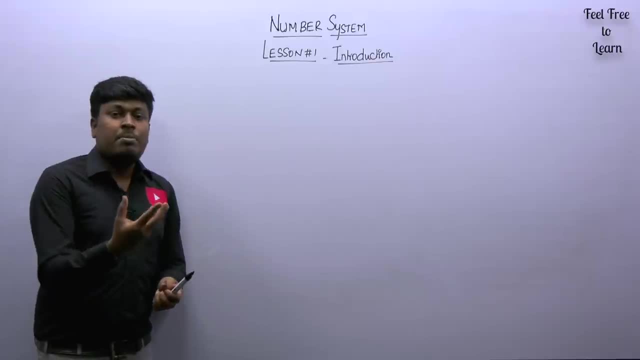 system. So, friends, listen here. instead of spending more number of time on biarting the concepts, better you can understand this chart, what I'm going to teach now. If you understand this chart, then you can save more time on biarting the concepts. So now let's move on to the chart. 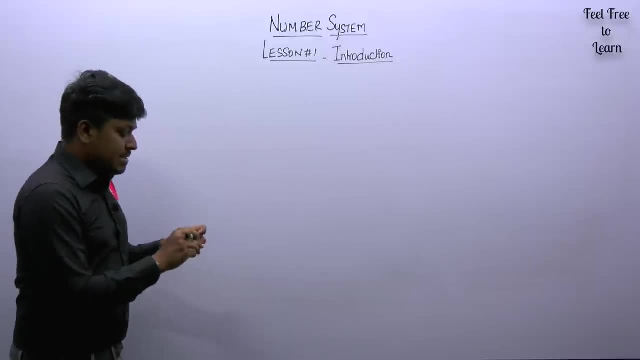 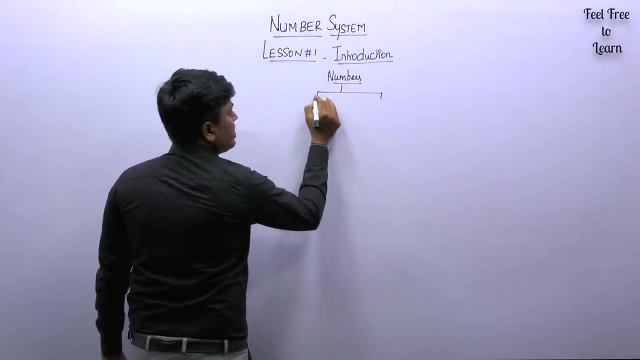 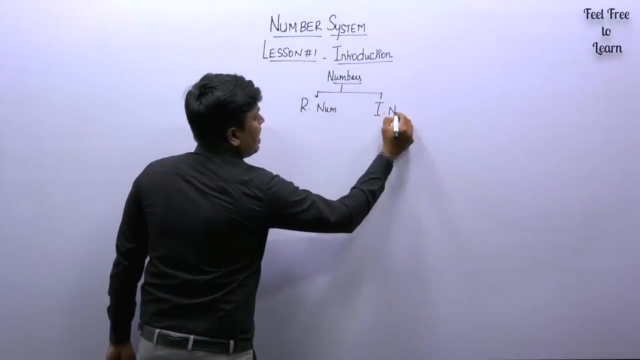 more number of time instead of biarting it, It is easy, right? Just see here. First let me take numbers. So numbers is basically separated into two categories. So category number one will be real numbers, Got it? Category number two is imaginary numbers. So numbers are separated. 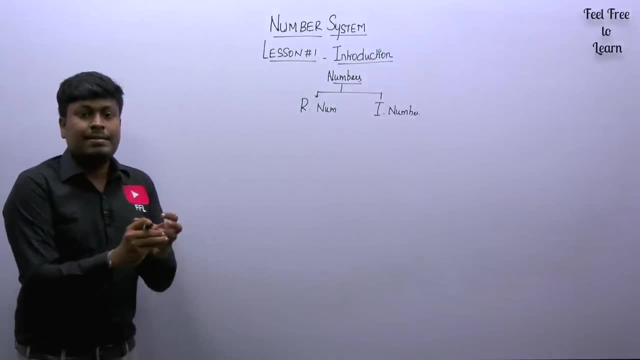 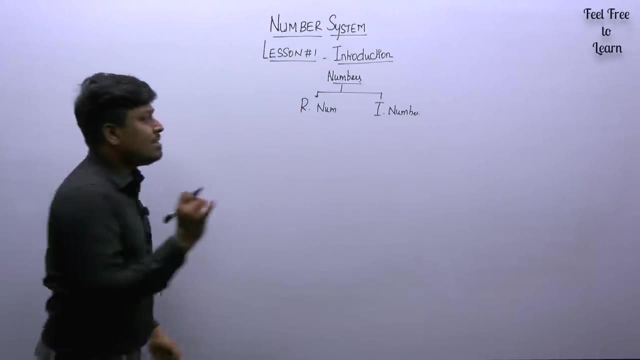 into two parts. One is a real number and the second is the imaginary number. So first you need to know what is called as a real number and what is called as imaginary numbers. Just see here numbers. let me take example: four plus three, i Got it Four plus. 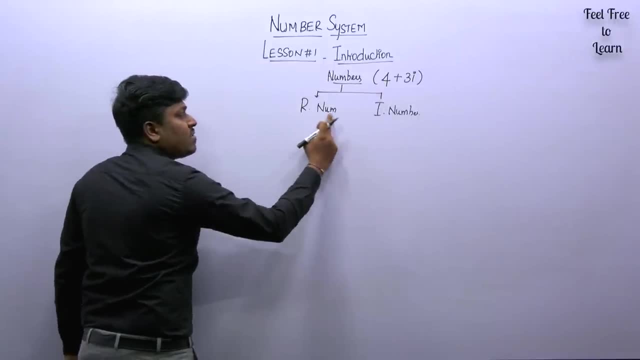 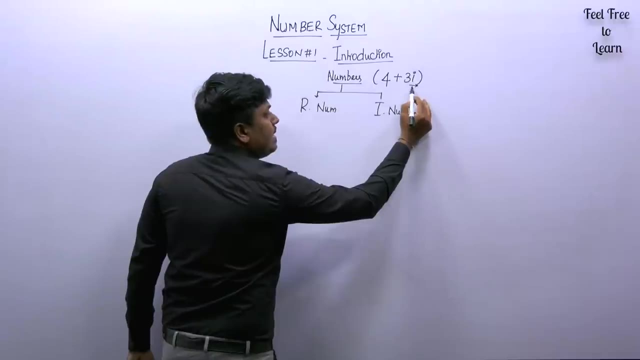 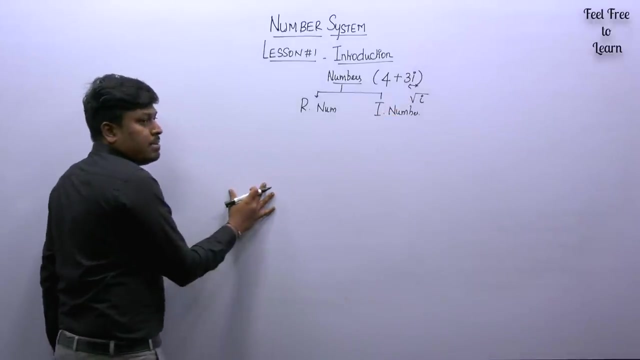 three, i Here. four is a normal number which is called as a real number. Imaginary number is like whenever you can able to see that letter i. sometimes you can able to see root of i. Root of i is minus one, So these cases is called as imaginary numbers, If a number contains a letter. 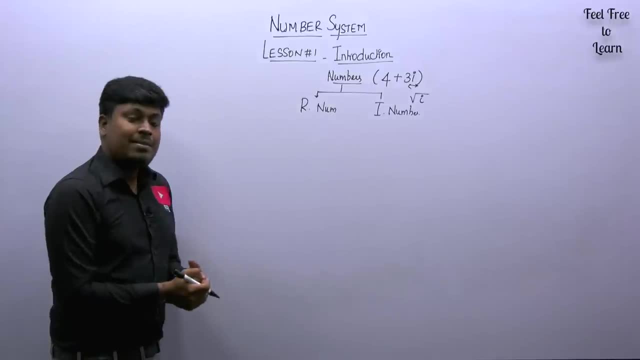 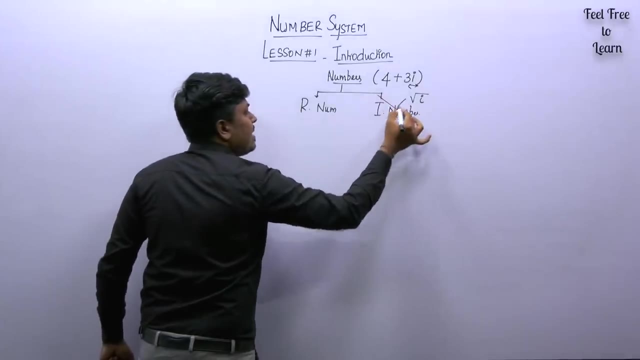 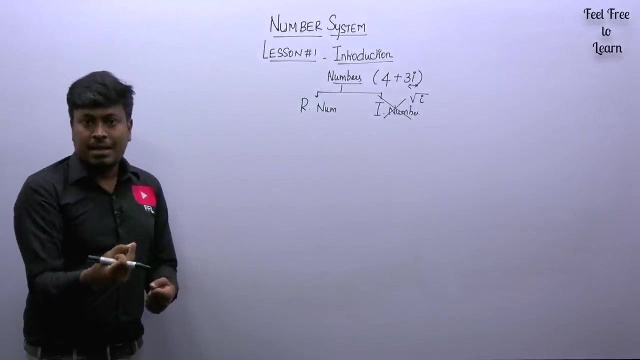 if a normal number is called as a real numbers. Just see, here we are preparing for competitive exams. In the competitive exams 99% imaginary number questions will not be asked Only if you are preparing for 9th standard, 10th standard or engineering mathematics. there we can able. 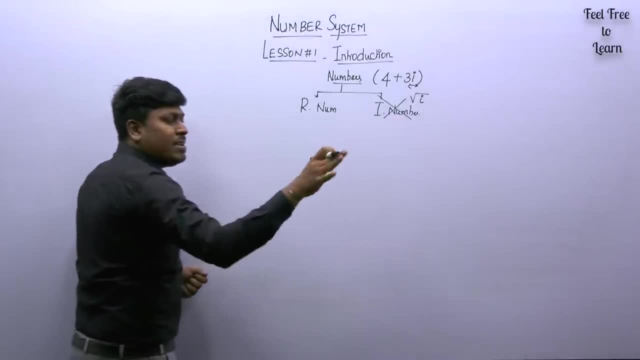 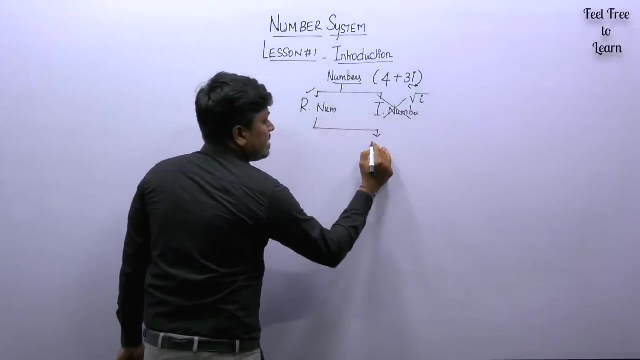 to see more number of questions on imaginary But in quantitative aptitude. you don't want to learn this. imaginary number concepts right. You can concentrate only on the real numbers, Got it? Second, this real number is categorized into two parts. One is irrational numbers. 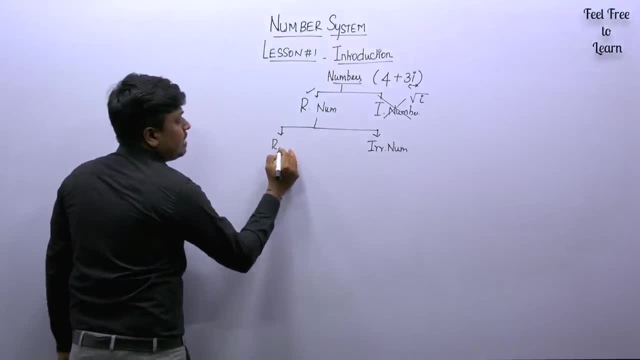 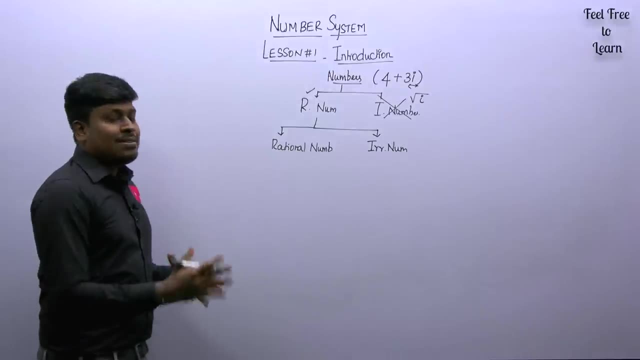 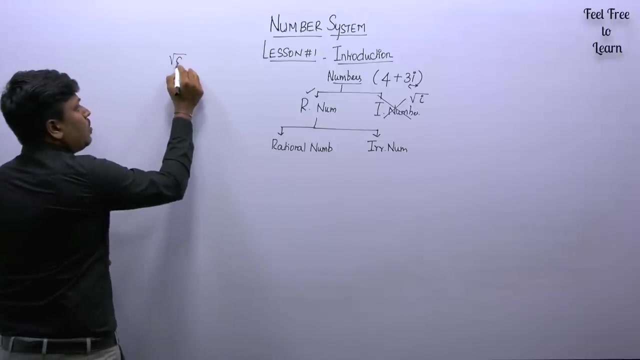 Got it. And the second is the rational numbers: Rational numbers and irrational numbers. So let me understand what is called as a rational number and what is irrational number. Just see here: what is root of nine? Root of nine is three, Yes or no? What is a root of nine? 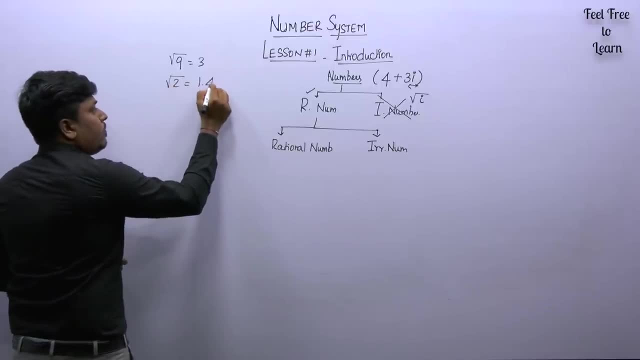 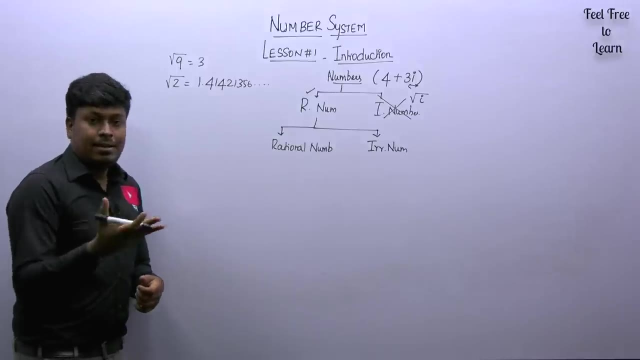 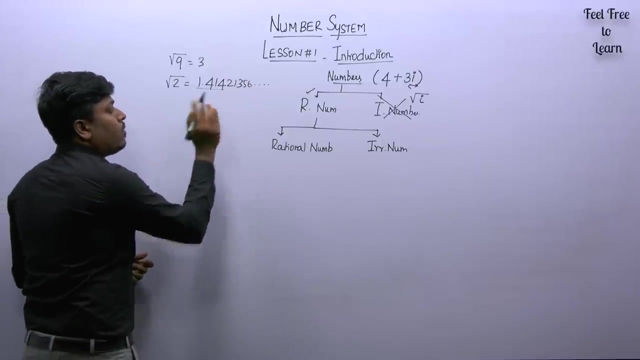 Root of two. Root of two will be 1.41421356.. It goes on, Yes or no. When you look at the calculator. just check the calculator. What is square root of two? If you find what is square root of two, we have learned only 1.414.. But actually the square root of two is 1.41421356.. 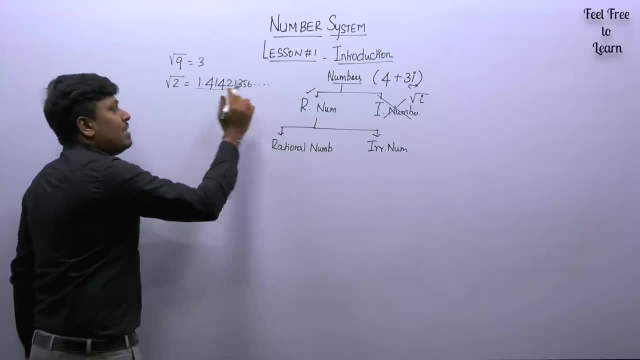 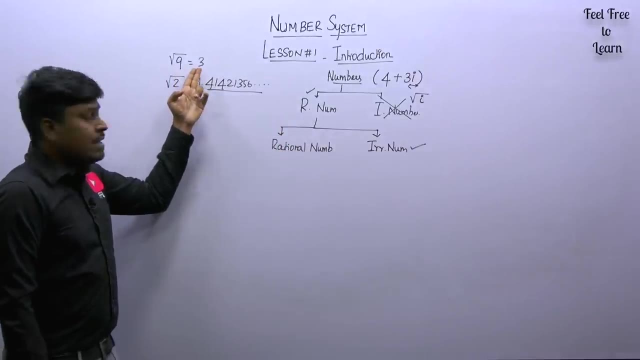 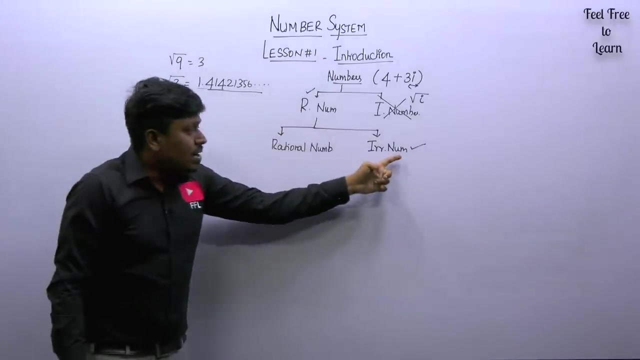 It goes on. It does not have an any end. So these cases are called as irrational. So got it Only if it is root. nine is three, Right, This number has an end, But this number does not has an end. So if a number that does not has an any end is called as irrational, 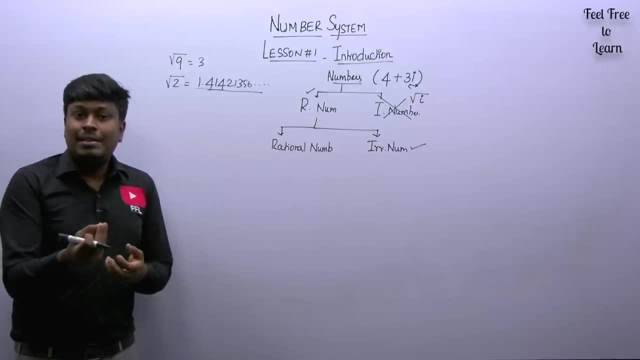 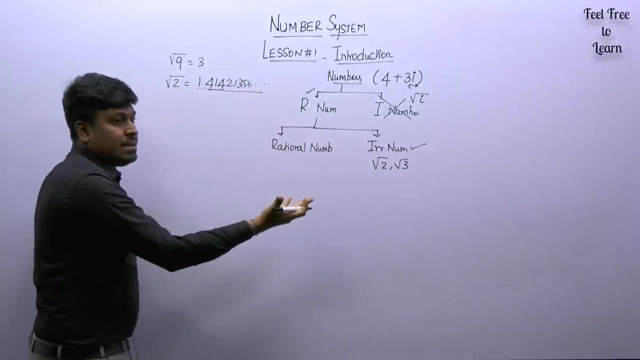 numbers, For example, root two, root three. So these are the numbers: Yes or no. Root two, root three. These are the numbers that does not have any end after the decimal point. So these numbers are called as irrational numbers, Right? So these are the small, small. 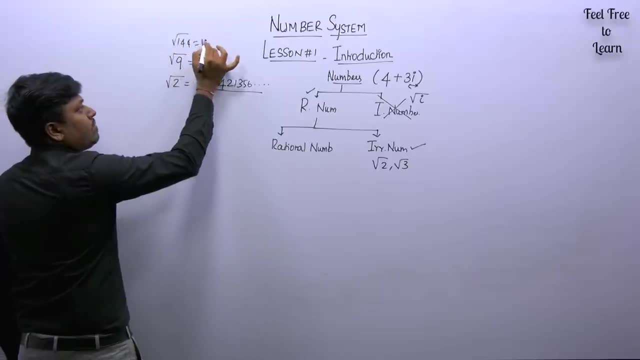 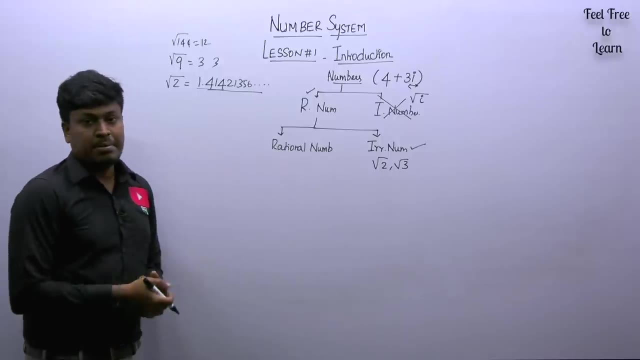 numbers. For example, a root of 144 is 12.. Yes or no, And normal number three, normal number four. it has an end. So these numbers are called as a rational, numbers Understood. So now we have learned what is called as numbers, how it is separated into two types. So in 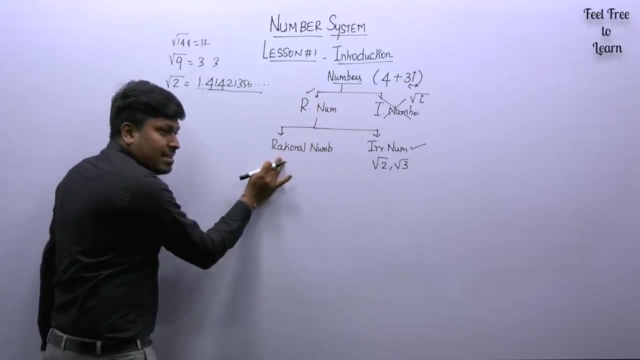 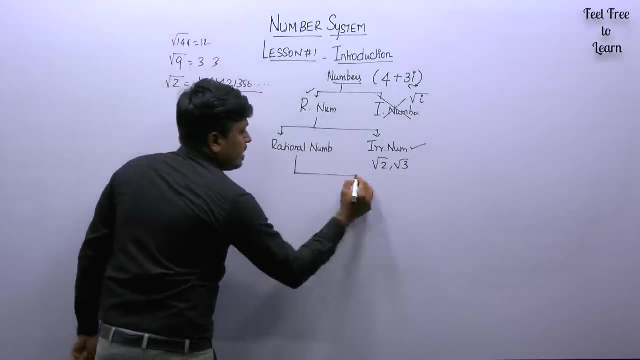 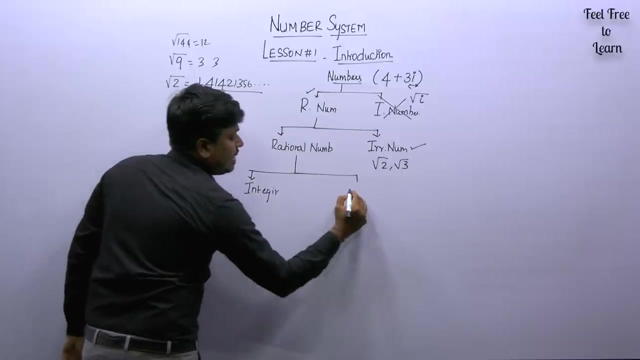 the real numbers. we have two type: One is called as a rational numbers and the second is called as irrational numbers. Got it Next? this rational numbers are separated into two parts, See One is the integer and second is the fraction. It is easy, What is called as an integer? 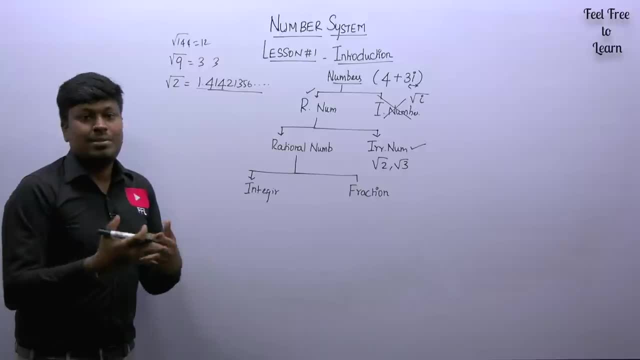 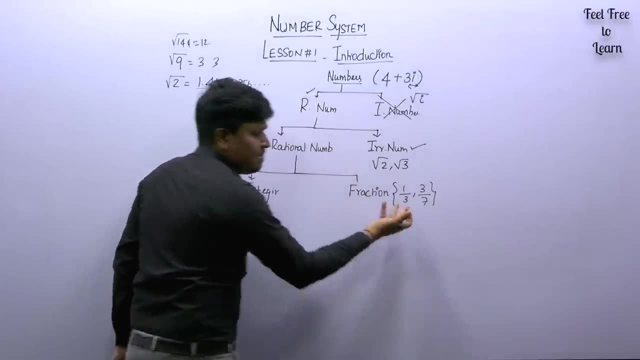 Integer is a normal numbers. For example, one, two, three, four. This is called as an integer Fraction. it is easy, Right? So one by three, three by seven, No fraction numbers. This is the fraction numbers, Got it? So this rational numbers are separated into two categories. 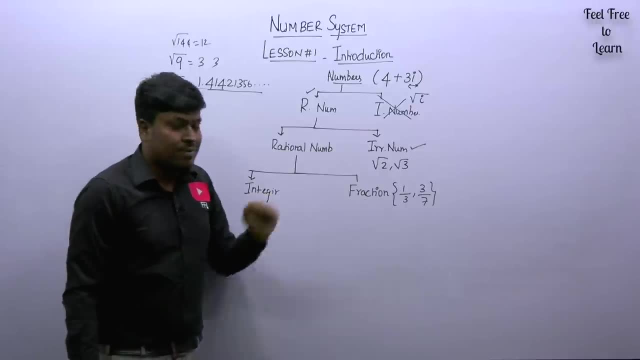 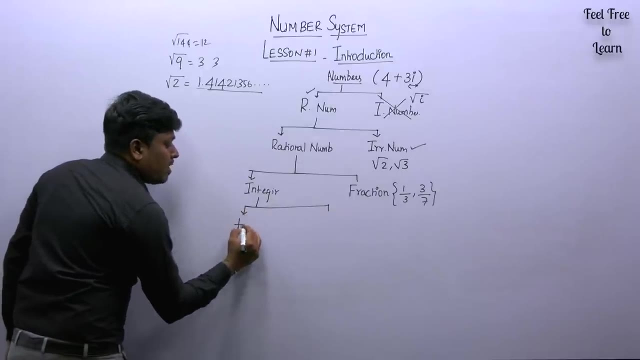 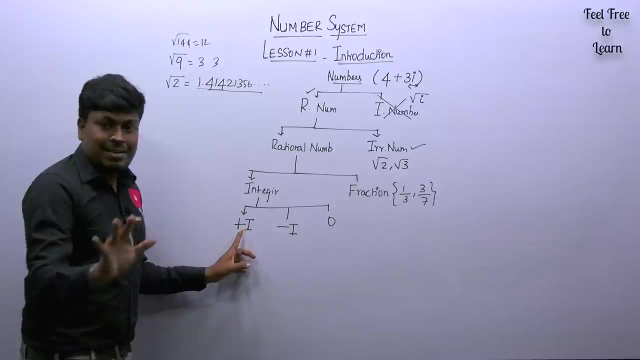 One is a normal integer and the second is the fraction numbers. If you take this integer, this integer is separated into, for example, positive integer, negative integer and a number zero. See: positive integer is nothing but one comma, two comma, three comma four till n. It is called as a positive integer. Negative integer is minus. 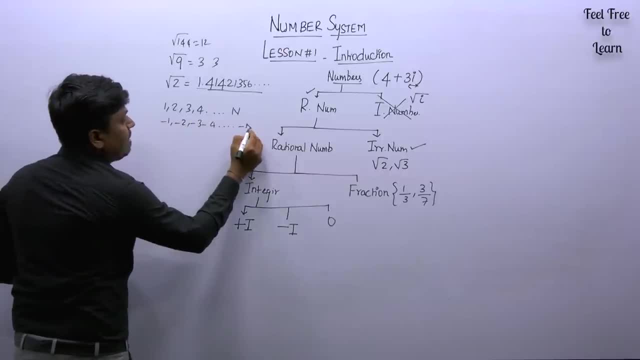 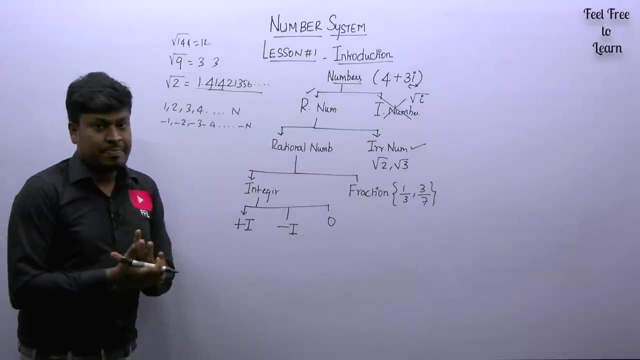 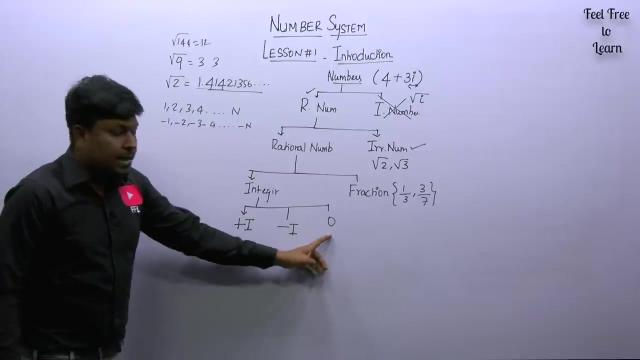 one comma minus two, minus three, minus four, It goes on till minus n. It is called as a negative integer. Zero is a normal numbers starting number, zero. So this is zero. So this integer is separated into three categories: Positive integer, negative integer and then zeroes. Got it, So now let 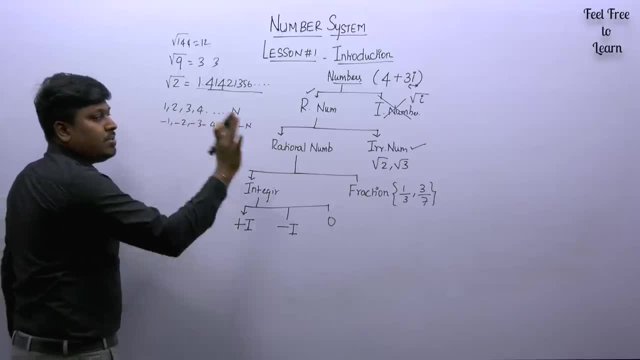 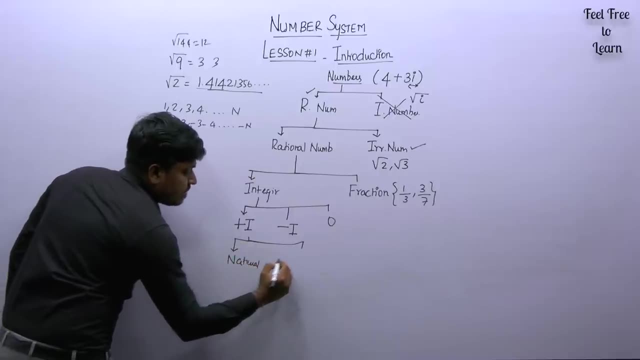 me take this positive integer. Positive integer is what one, two, three, four. So this positive integer is categorized into two parts. One is the natural numbers. Second is the old number. Everyone knows it, what is called as natural numbers. 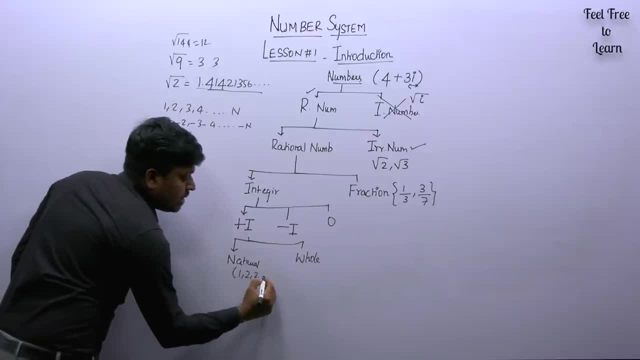 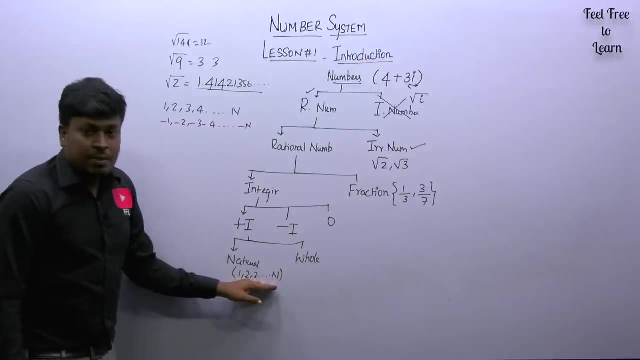 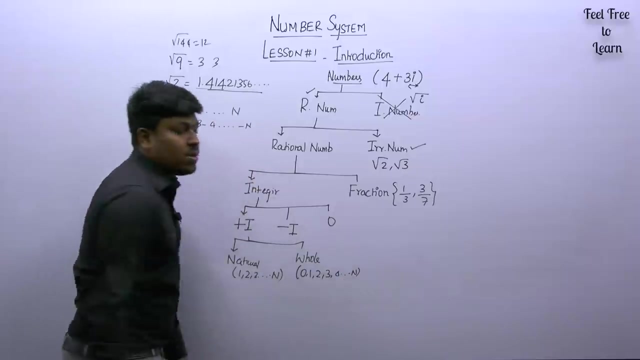 And numbers that start from 1, 1 comma, 2 comma, 3 comma, 4 until n, it is called as natural numbers. What is called as old number? A same set of series. if we start from 0, 0 comma, 1 comma, 2 comma, 3 comma, 4 until n, it is called as old numbers. 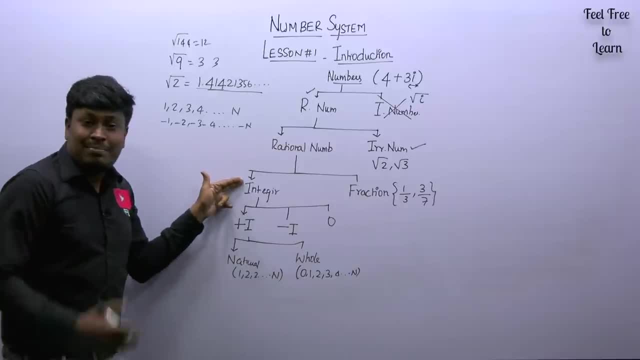 So friends got it. Just see here integer is separated into. it is subdivided into three parts: positive integer, negative integer and a 0. You know what is called as integer. Integer is a normal number: 1 comma, 2 comma, 4 comma, n. 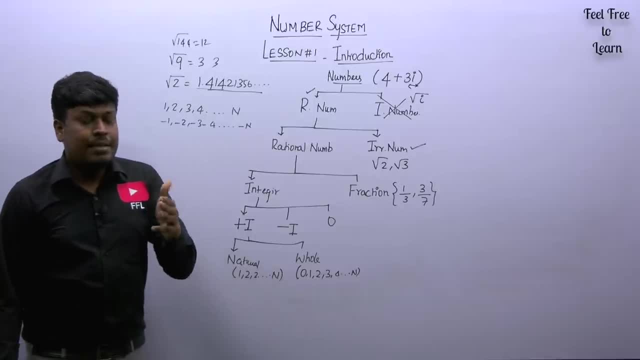 So we have integer two type: positive integer, negative integer and a number 0. So if you take a positive integer that can be separated into a natural number and a old number. Natural number is nothing like a series that start from 1, it is called as natural number. 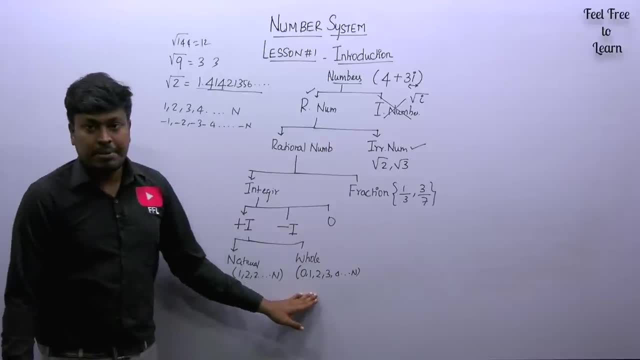 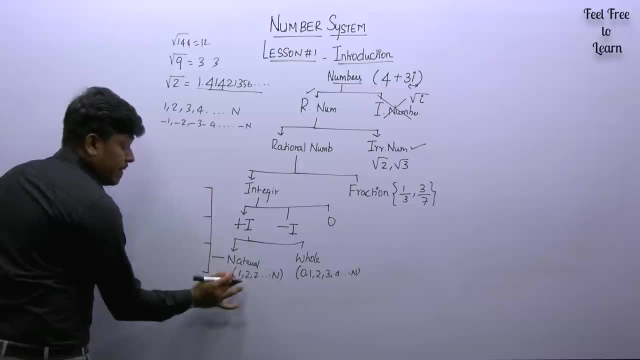 If a series that start from 0, it is called as a old number- Got it The last step. This natural number is separated into four important. there are many parts, but I am teaching you only four important parts that are important for competitive exams. 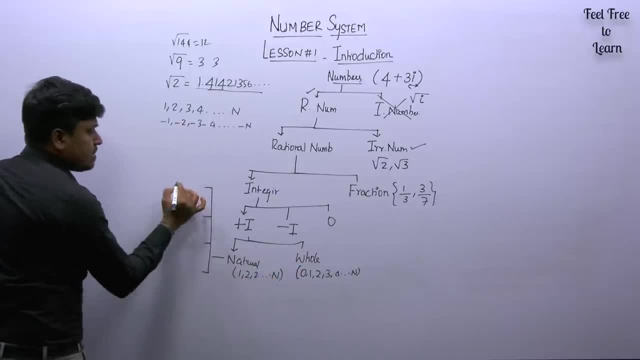 So 1 comma, 2 comma, 3 comma 4 till n, How you can separate this? Even numbers: Yes, even numbers. 2,, 4,, 6,, 8, even numbers. Second will be odd numbers. 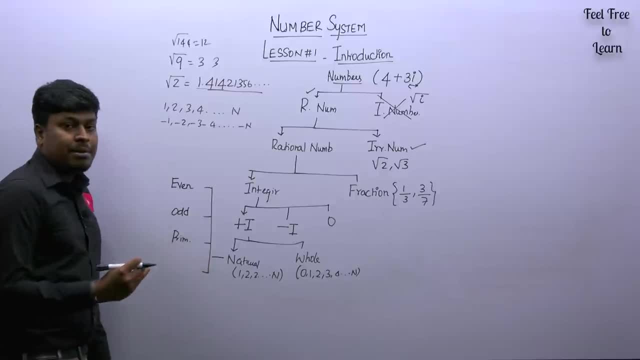 Third will be prime numbers, Yes or no? What is called as prime number? 3,, 5, 7.. Those cases are called as prime Prime numbers. And the last is the composite number. You should know what is called as composite number. 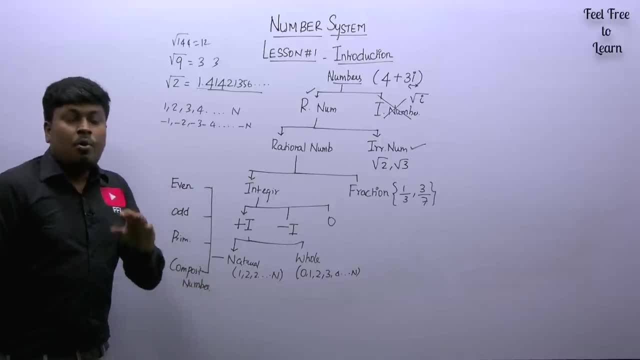 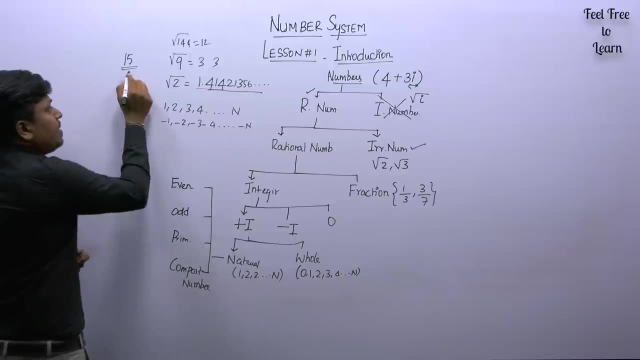 Composite number is a number which have more than two factors. For example, let me take number 15.. How many factors we have? 5 into 3 will be 15.. One factor, 3 into 5, will be 15.. 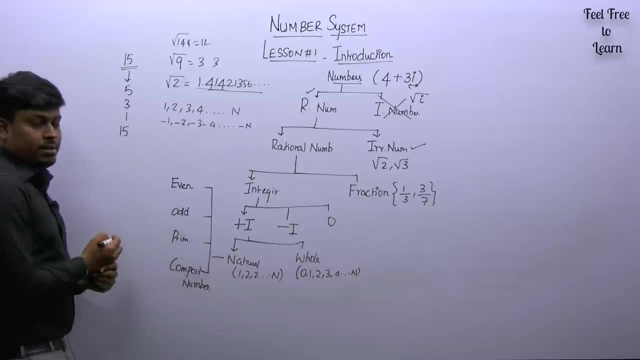 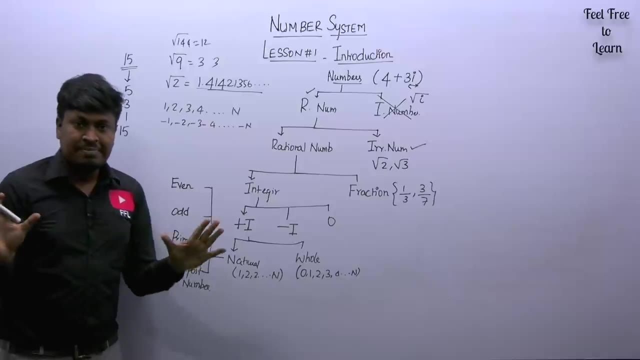 1 into 15 will be 15.. 15 into 1 will be 15.. So if a number which has more than two factor is called as a composite, Then you have a composite number. That's it, Right. 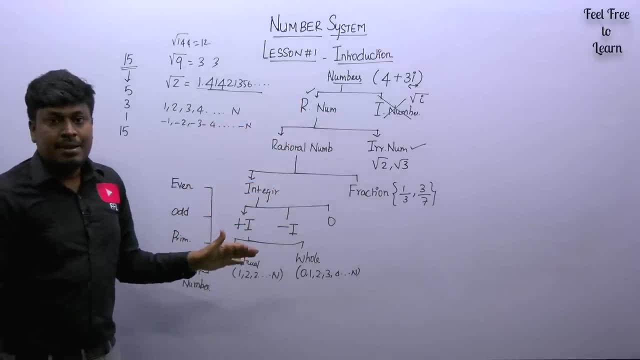 Just see how easily we have categorized the number system. And now, without bias-getting it, it is easy to understand the entire concept. Again, I'm saying there are more important points other than this, But I'm teaching only for the exam point of view. 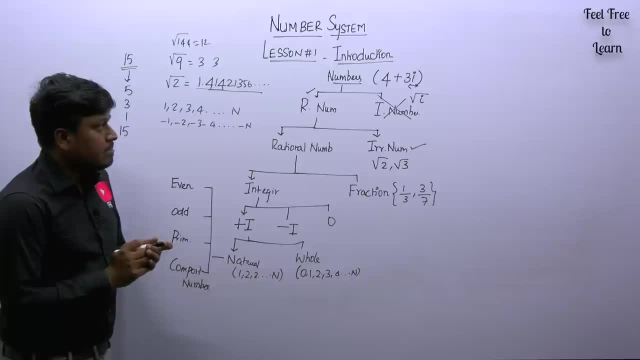 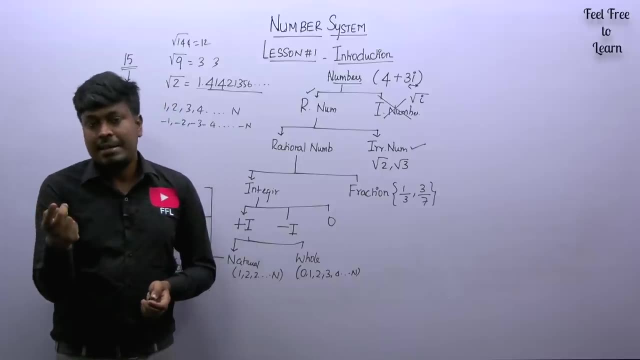 For the exam, competitive exam point of view. I can teach you again one time. See first numbers. Numbers are separated into two categories. One is a real number and second is the imaginary numbers. So real number is a real number, is the normal numbers. imaginary number is the number that contains i letter. i is called as: 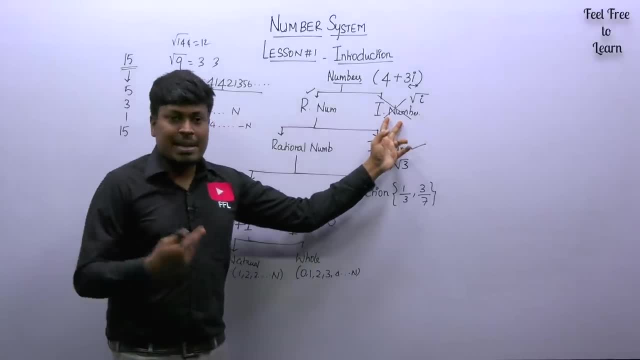 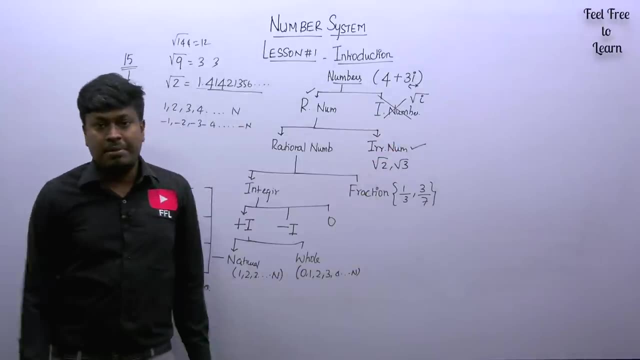 imaginary numbers. so you don't want to concentrate on more on imaginary numbers, because only if you are preparing for school, colleges, those cases we have to learn this. imaginary numbers for the competitive exams, quantitative aptitude. so this real number is more than enough. second, the real number is categorized into two parts. one is a rational number and the irrational number i have 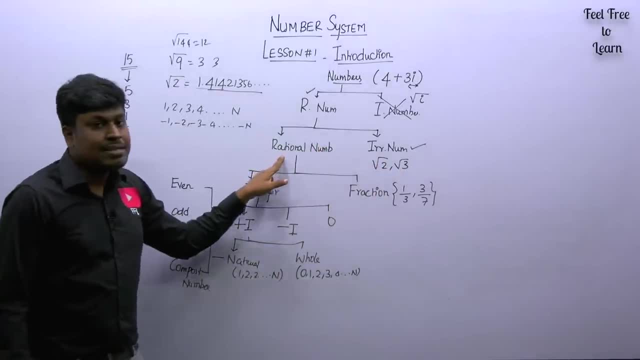 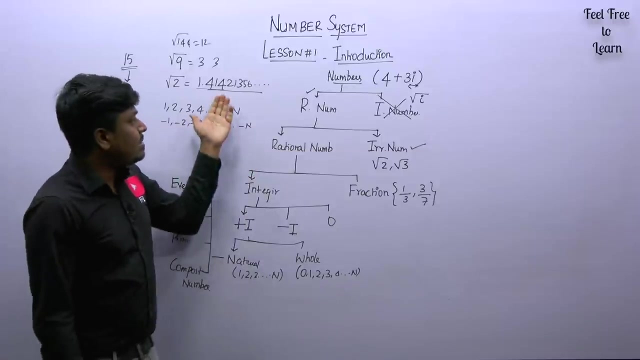 told you what is the difference between irrational numbers and the rational numbers. if a number that does not have an end, it is called as irrational number. example: square root of 2. if you find what is the value of square root of 2- 1.41421356, it goes on right. so those cases is called as an 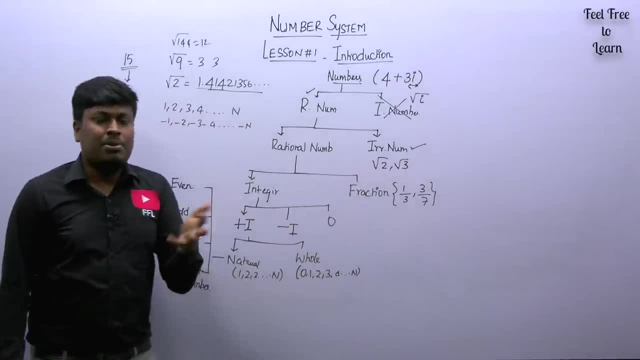 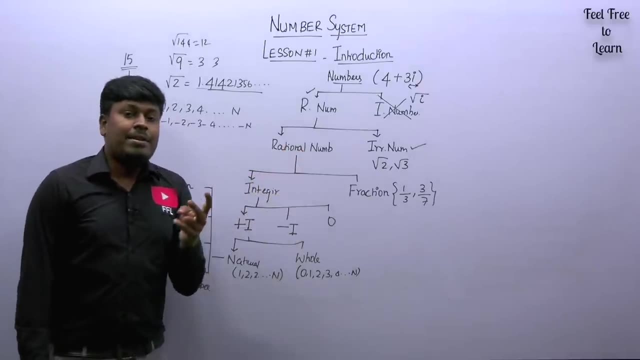 irrational numbers. so rational number is like normal number: root of 9, 3, 4, 5, etc. got it. so now this rational numbers are separated into two categories. one is a normal integer and second is the fraction. fraction, everyone knows: 1 by 3, 2 by 7.